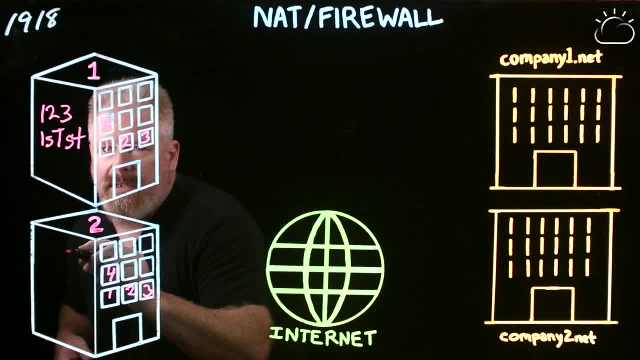 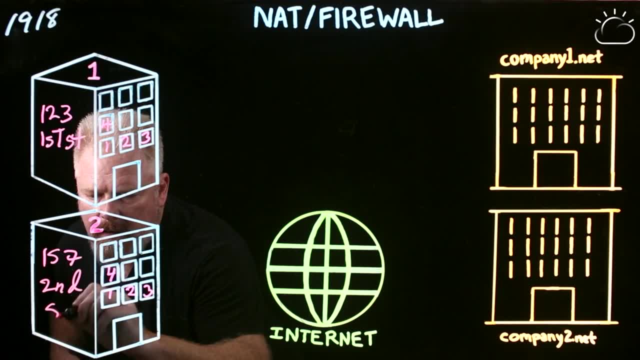 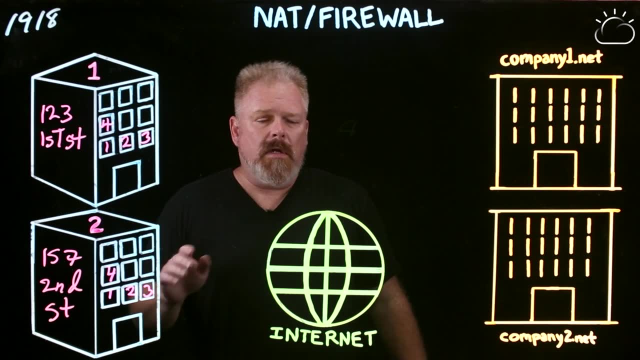 and apartment 2 is 157 Second Street. Okay, so those addresses, the street address, is uniquely addressable across the world, whereas the apartments themselves, the apartment numbers, are not unique. So that really describes the difference between an internal 1918 TCP IP address and an external address Well. 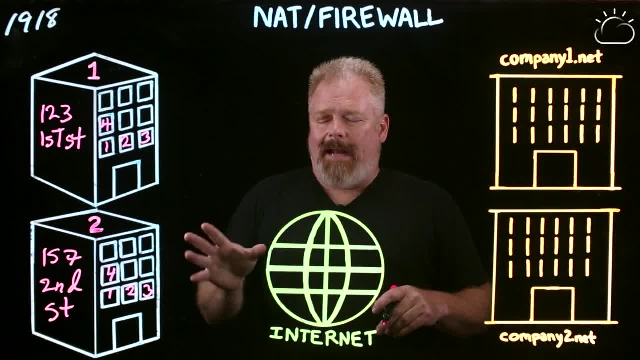 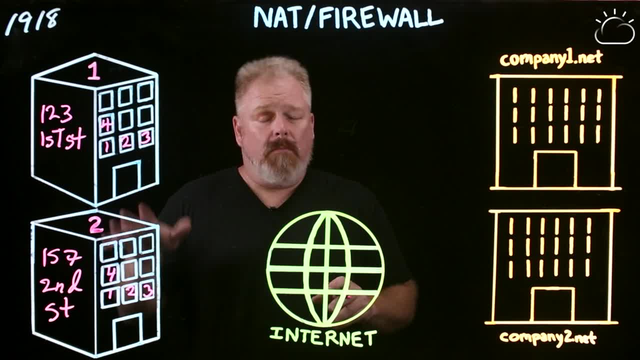 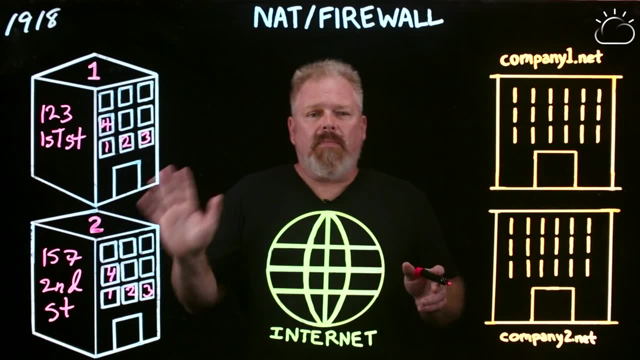 how do you get between those two things? You get there by something called NAT, network address translation. NAT is typically used to translate an IP address from one range or multiple IP addresses from one range to an IP address on some other range. It's commonly used between private internal 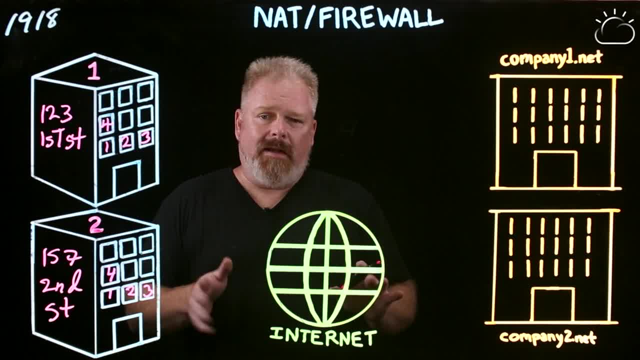 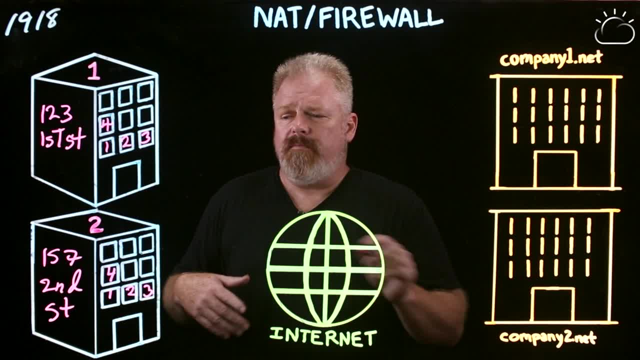 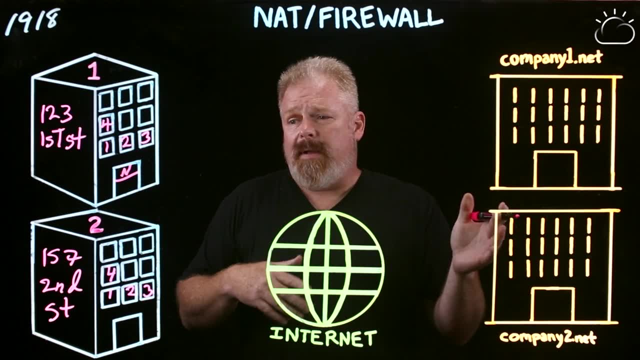 networks and an internet IP address, because those are finite And subsequently they can be very expensive to purchase or to use, right. So in the case of apartment 1, we have a device that does our NATing, And the second part of this topic is firewalls. A NAT device typically goes along with a 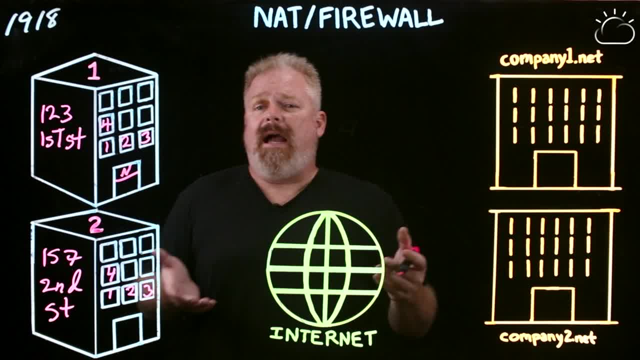 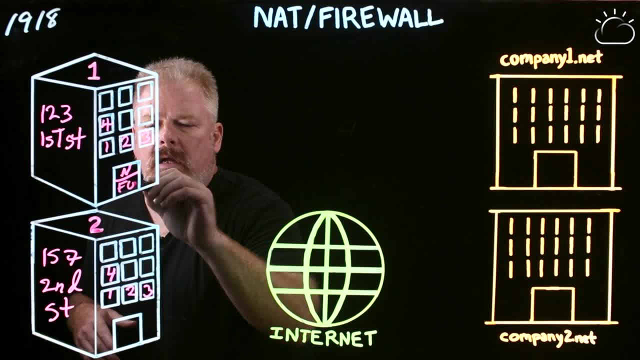 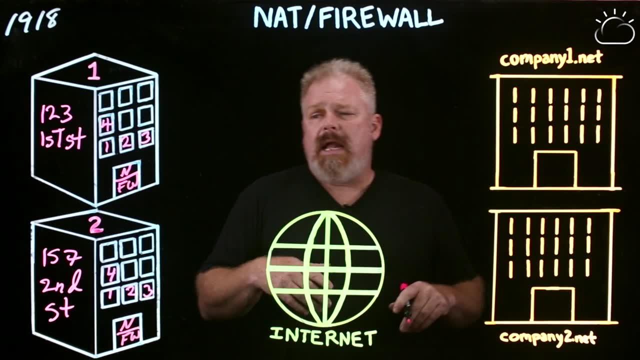 firewall function and it's usually employed in some kind of a routing device. A routing device connects two or more computer networks. So we're just going to put our firewall down here in both our apartments here. So NAT firewall. Okay, so let's say someone in apartment 2. 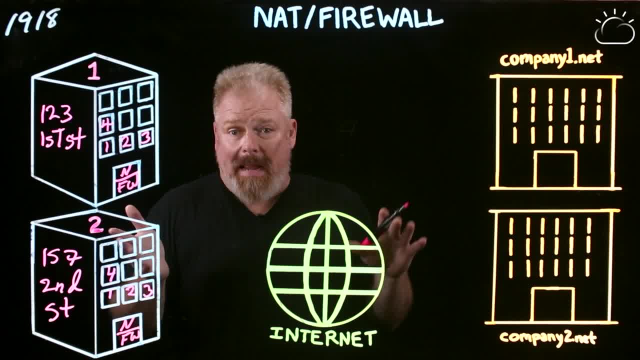 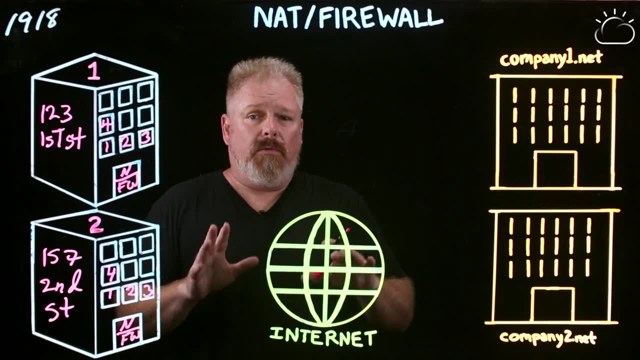 wants to communicate or send a letter, a mail- remember those Mail- over to company1.net and he wants to send it out over, you know, from his street address to the company 1 street address, Or let's just say from his internal IP address to 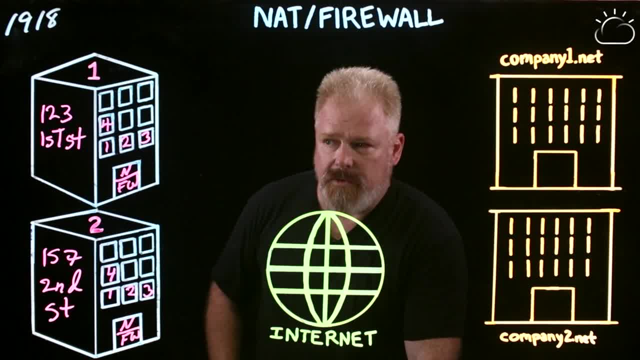 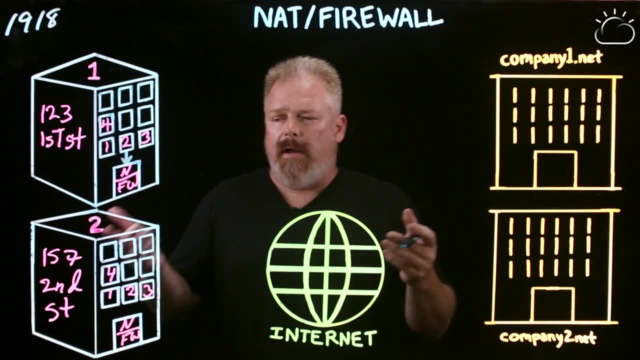 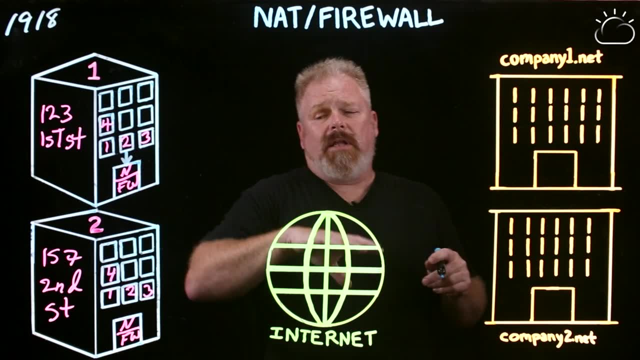 a public IP address or an internet IP address. What he would do is send that out to the NATing device, which is akin to: let's say, you have a home router or a routing device. That's the first device. your traffic's going to hit The NAT network address. translation part of that is going to: 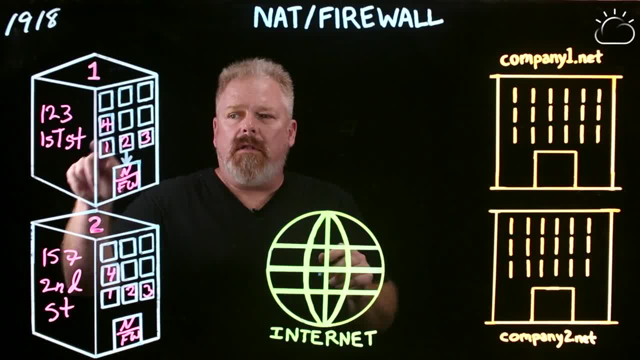 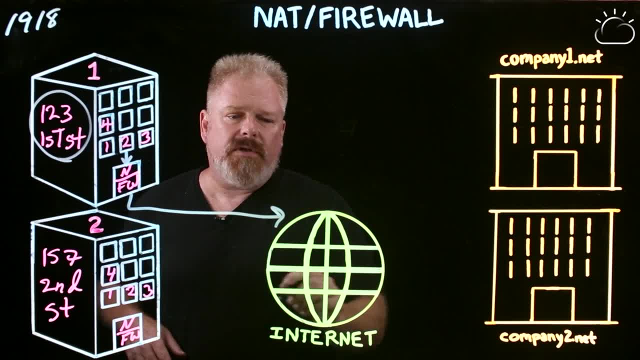 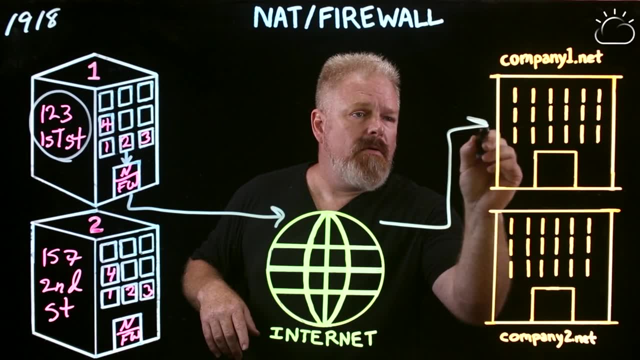 convert that internal address to a real internet address, which is what It's- this 123 1st Street. That traffic is going to traverse from 123 1st Street, so it's like sending a mail with the return address being 123 1st Street over to company1.net. As soon as company1.net sends a response, it's. 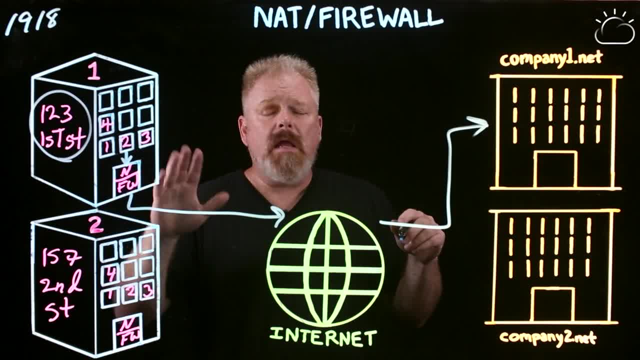 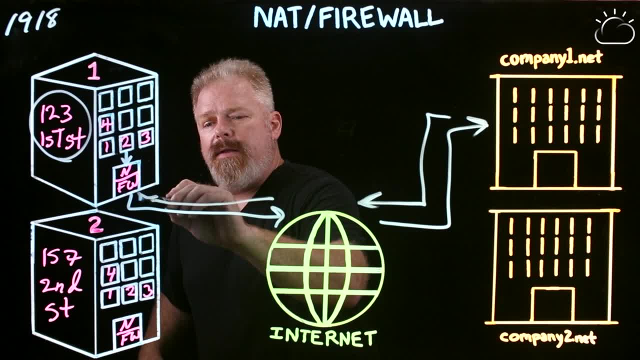 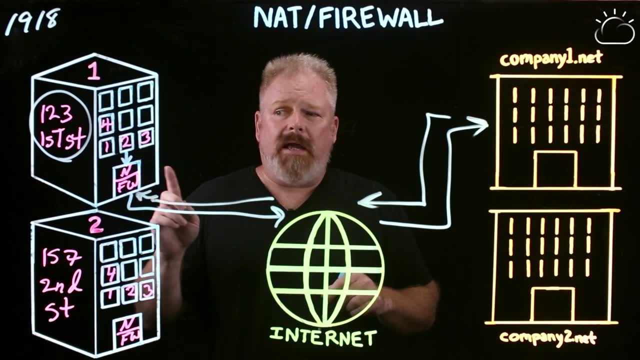 going to not send it to apartment 2,, it's actually going to send it to 123 1st Street. All right, it's going to send a response back and what's going to happen is the NATing device actually keeps track of what's going out and the corresponding response And it. 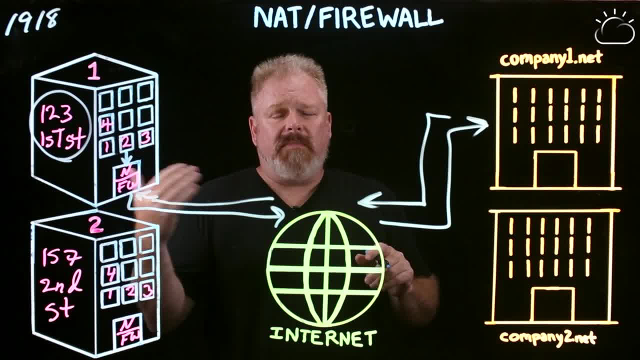 knows that the response to 123 1st Street- let's say it's the person who's going to deliver that card to apartment 1.But let's say it was his real name and it knows that that's a given address And when that person pulled this response. 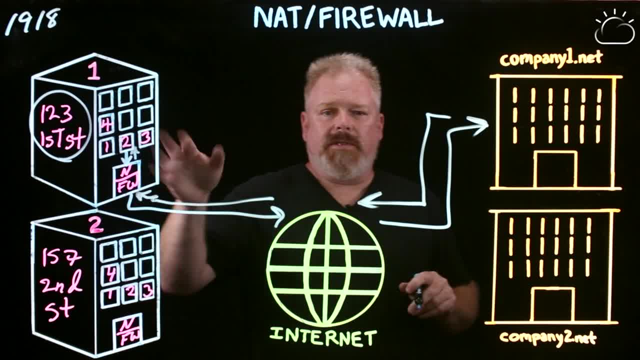 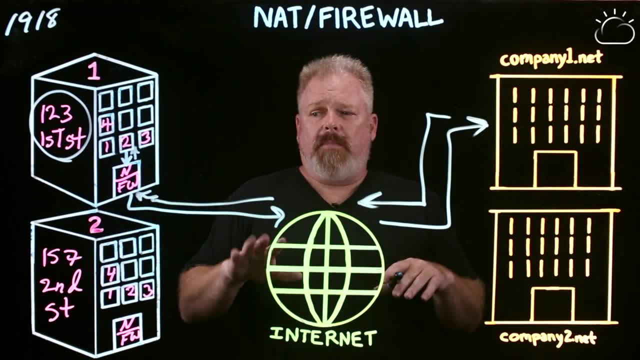 on because it's a given address that was sent to him by the department. it knows that his real name was going to be in the person's name. They put their name on the letter going out. it knows it converts that to an internal address. 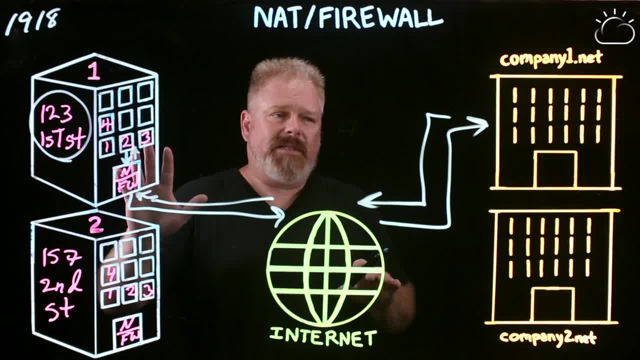 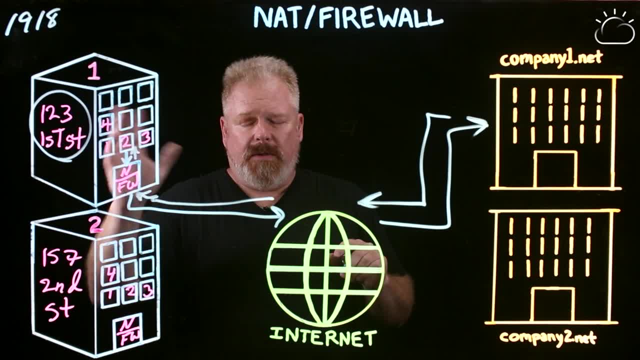 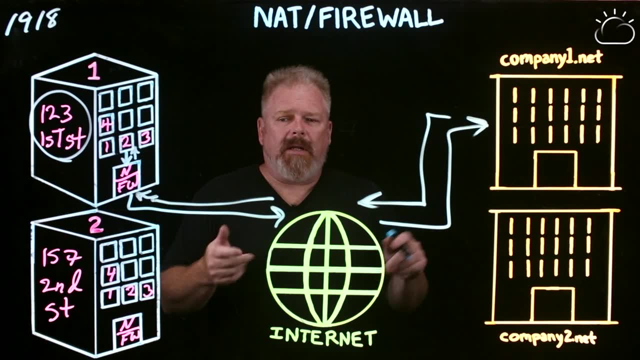 which happens to be apartment 2.. It knows that person lives at apartment 2.. Here's the key: Company 1 doesn't know that that person lives, And it's akin to a security device. Now that by itself is typically not enough. 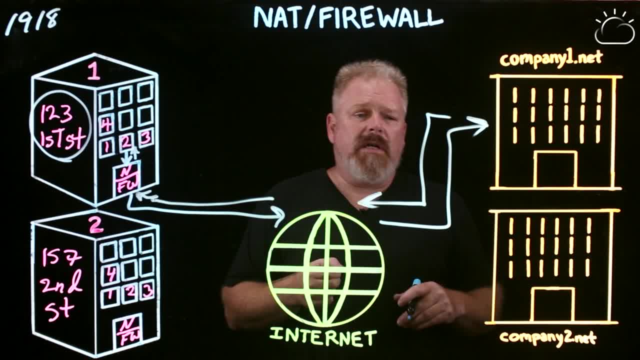 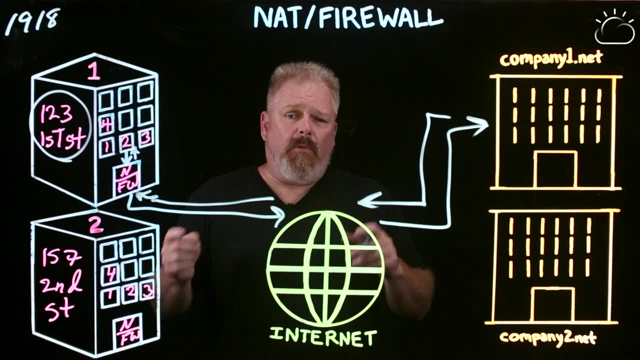 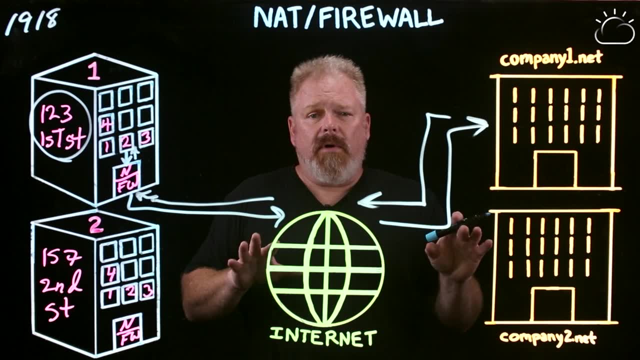 On the same device, we'll have a firewall function. What's a firewall function? A firewall function is known as a security device service appliance that actually monitors the network communication between some source and some destination, typically deployed across two different networks. 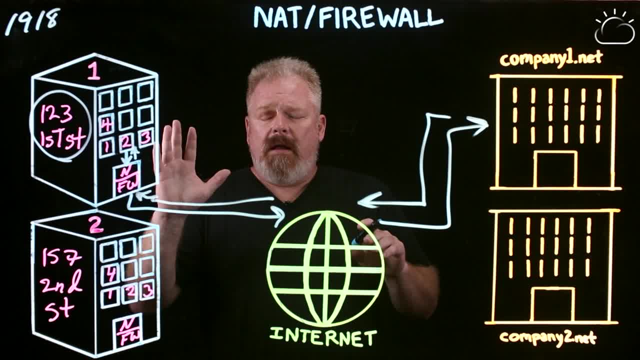 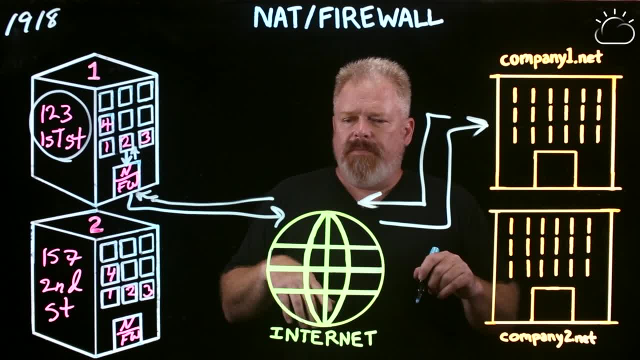 That's not always the case, but in this analogy we're going to just say the firewall is there between the internal network and the external network And notice, we have it deployed with our NAT device. So in a typical firewall we'll have something called. 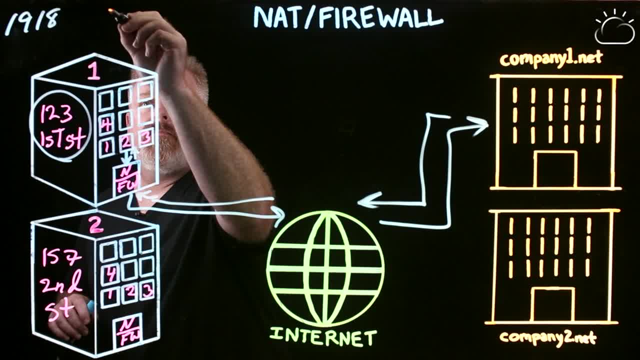 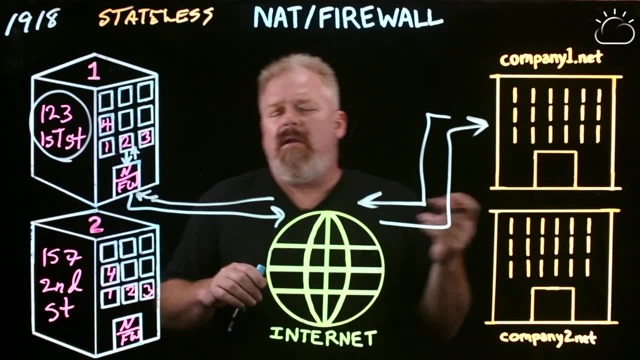 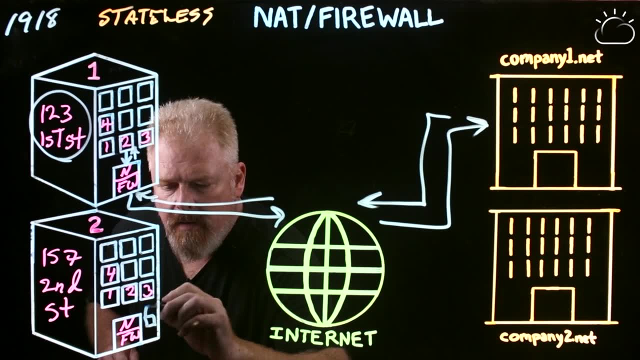 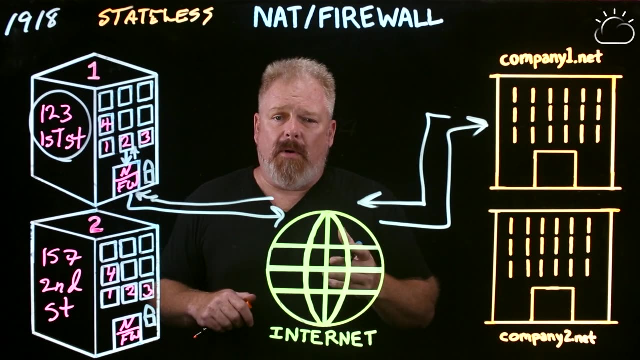 the very first firewall, something called a stateless firewall, And all the stateless firewall is. it's just like a lock on the door. So if we put a lock over here and we put a lock over here, all that says is: I'm a person that. 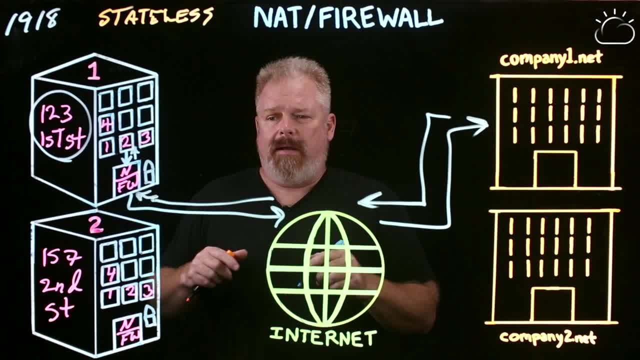 wishes to get into the apartment. I have a key. I'll open the door and go in. Well, it's not a bad way to go. It keeps most people out of the apartment building that don't live there, But somebody can tailgate and they. 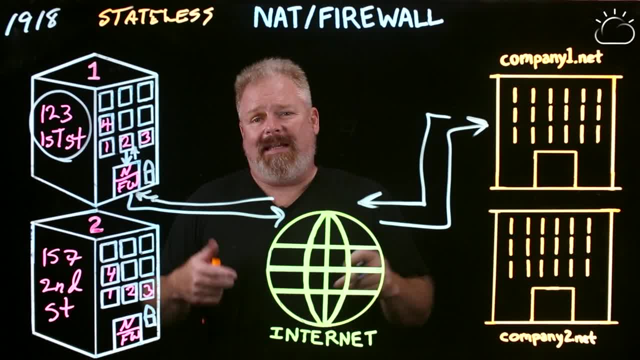 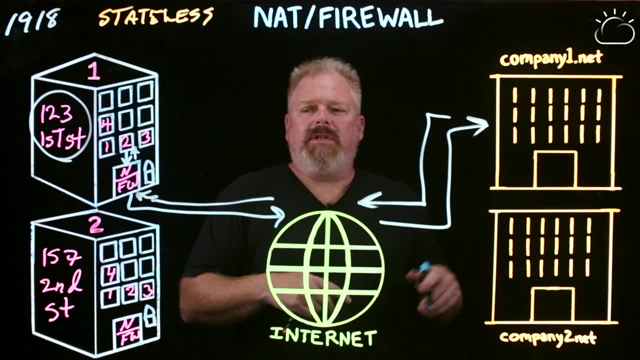 can go in behind that traffic. Maybe they figure out the key. There's a couple of different ways. It's a decent firewall, but as things get more sophisticated it's not enough. So the next type of firewall that came up was called stateful. 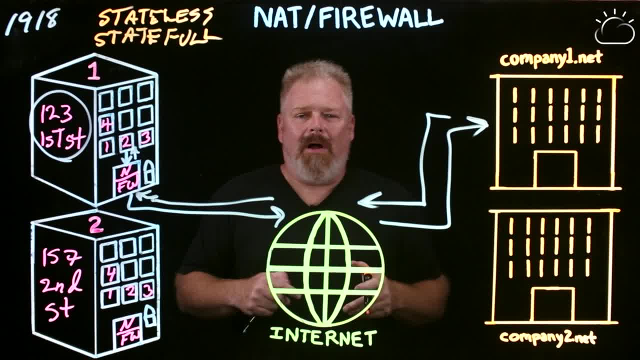 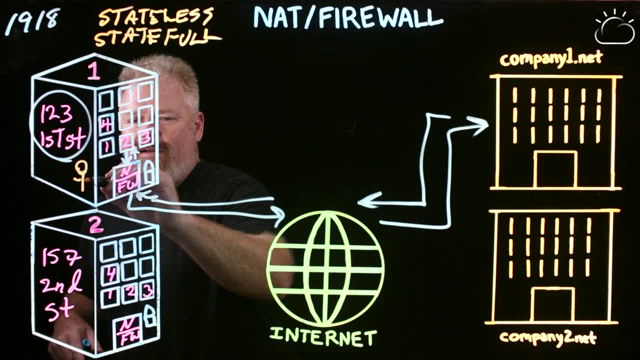 I love my writing, So a stateful firewall does this. Now we've hired a security guard. right, Here's our security guard. He's a cool dude. He's sitting at the front. He's sitting at the front desk. 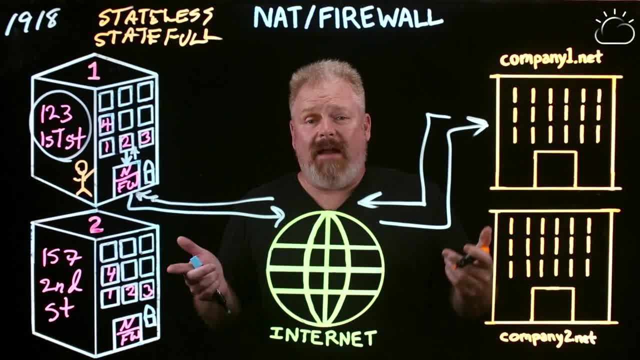 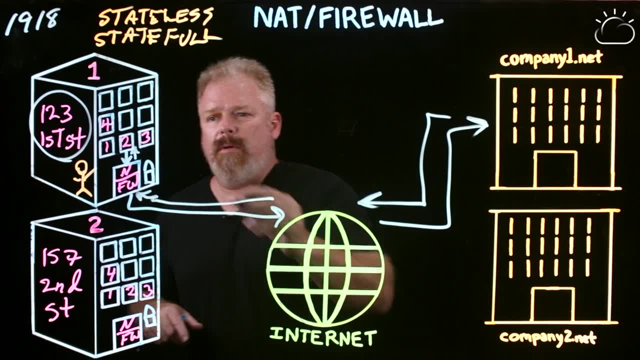 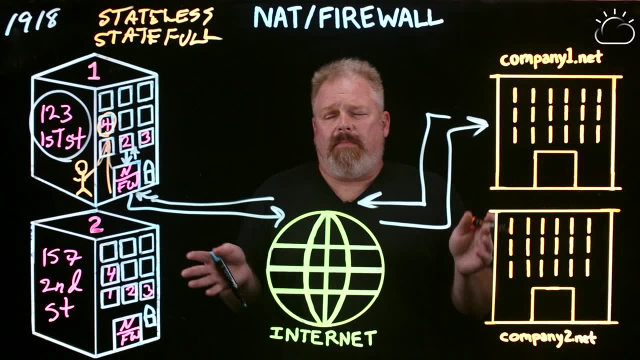 So as traffic tries to enter the apartment building- maybe they have a key- he looks at the person and says: where are you going? I'm going to apartment 4.. So, now that traffic's allowed, to apartment 4.. Doesn't ask what the person's doing there or anything else. 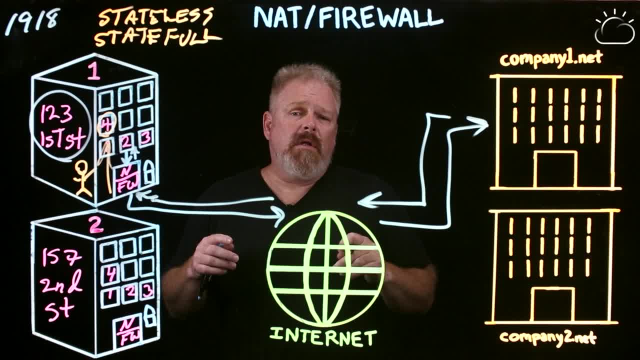 just allows the traffic. So really a stateful firewall will allow. understands the source and destination, It does the navigation of the traffic and it actually monitors the conversation between that source and destination and does a little bit more being a traffic cop. 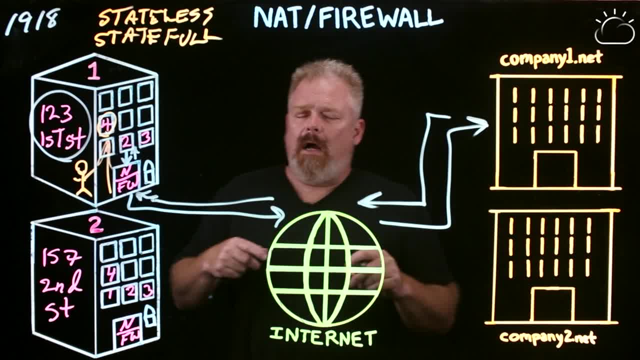 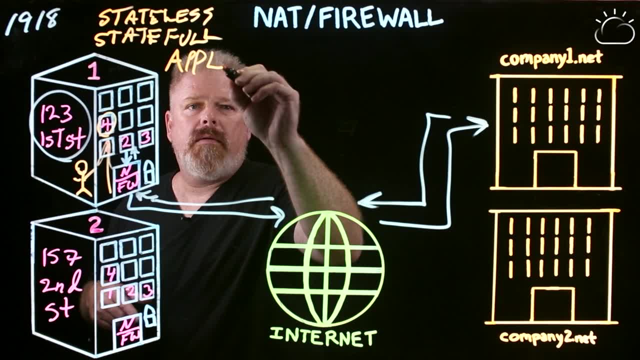 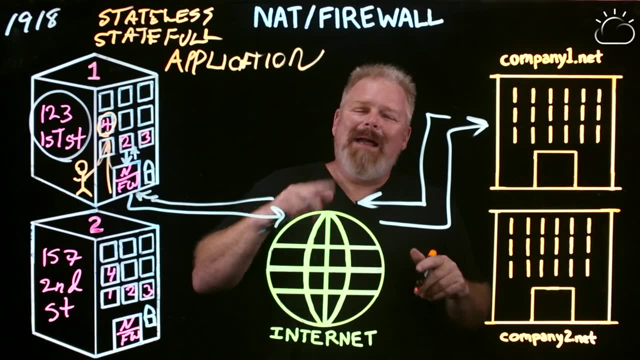 between those two source and destination. So last thing we're going to look at is something called an application firewall, And this is application Application, Application, Application Application. There you go. An application firewall is something that looks deeper at the conversation. 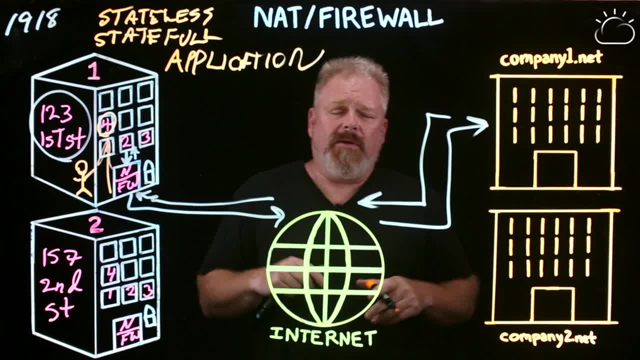 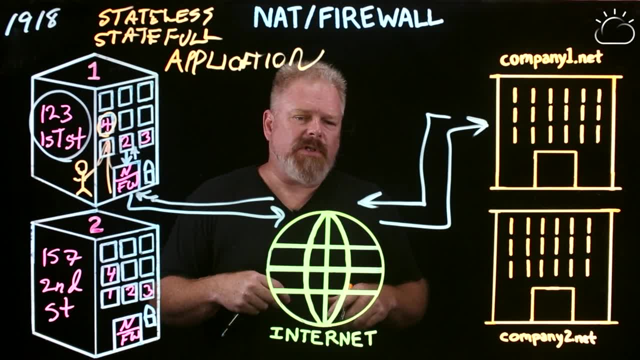 So now we have our traffic cop over here And what he's doing is now, rather than just asking what apartment you're going to, he's going to ask what your purpose is. So think of it this way. It actually looks deeper into the conversation. 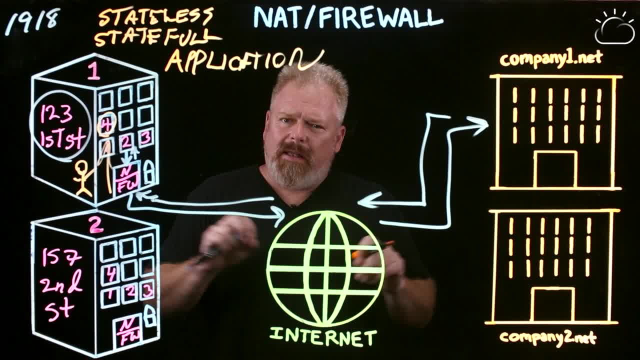 If we're talking about web service traffic, it makes sure that's really web type traffic, that's being communicated from the source and destination, Not just some other type of traffic that could meant to be, let's say, some kind of malicious traffic.